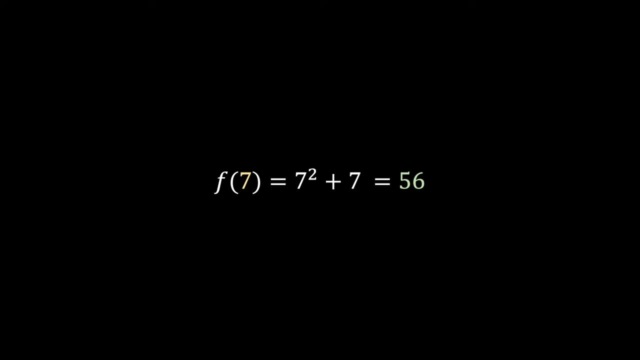 of seven, We will get 56.. Now the value of eight. We will get 72.. Now 20. We will get 420.. As you notice, this function expects us to be able to add x to the value of eight, So let's input the value of. 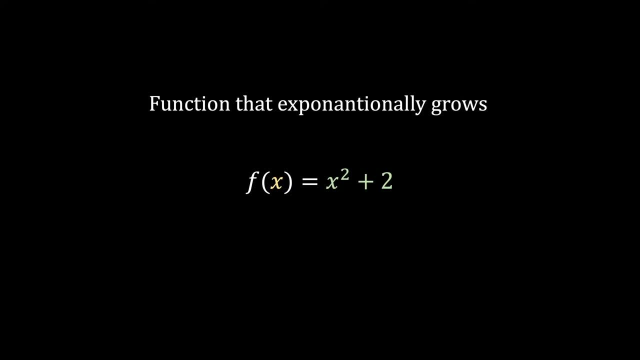 eight, We will get 420.. Now the value of eight, We will get 420.. Now the value of eight We will get exponentially grows. That means it grows quicker each time because we square x and scoring would make this function exponentially grow, with one exception. Let's show this function on a graph. 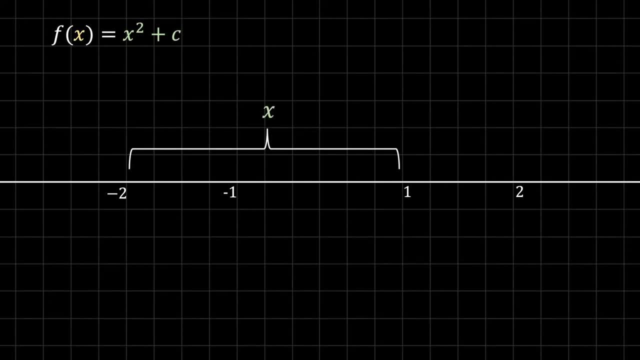 As you remember, I told you there was an exception to this exponential growth of this function, and that is, if we input these values between 1 and negative 2, the function would not exponentially grow because of the properties of arithmetic and algebra. So that means that the values as shown 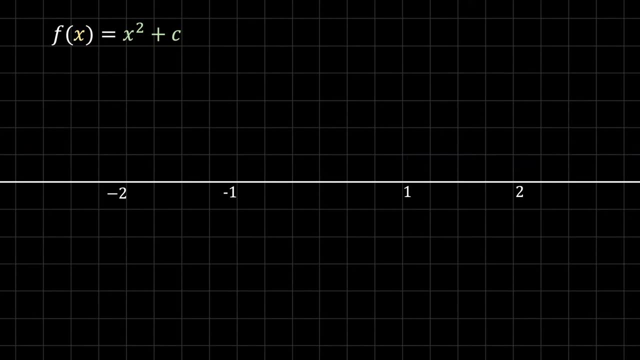 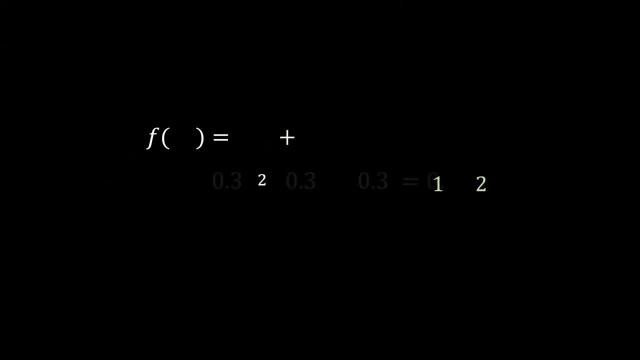 here would make the function exponentially grow, but the values between here would cause the function not to grow exponentially. Let's input some examples. If we input 0.3,, we are going to get 0.12.. If we input 0.1,, we are going to get 0.11.. How about negative 0.5,? you ask? We are. 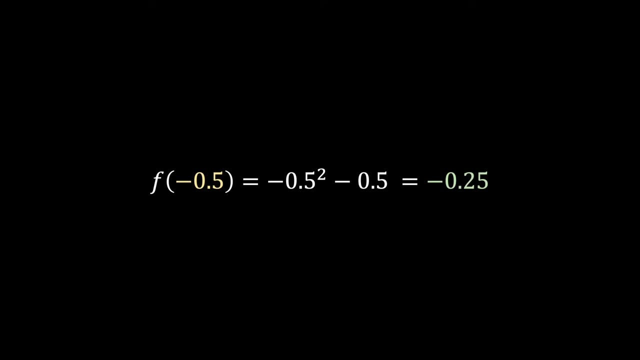 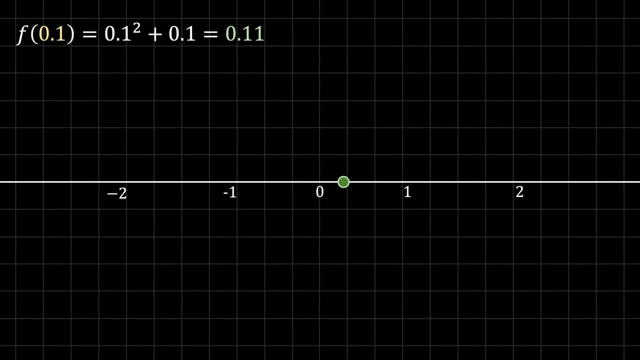 going to get negative 0.25.. Let's show these answers on a graph. Let's show the input of 0.1 on this graph. As you can see, it falls on the value of 0.11 as an output from this function. Negative 0.6, it would. 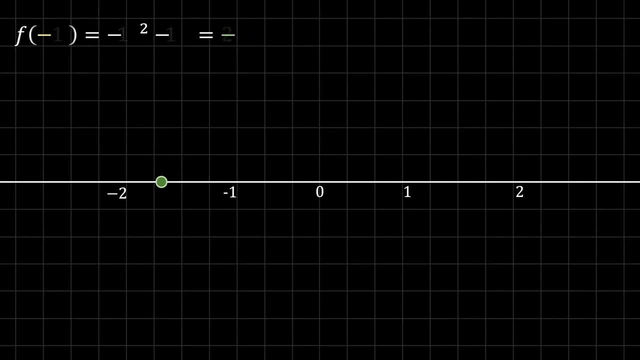 be negative 0.96.. Negative 1 would be negative 2, and negative 1.1 would be negative 2.31.. I also want to point out later in the video: all of the dramatic action will take place right here. 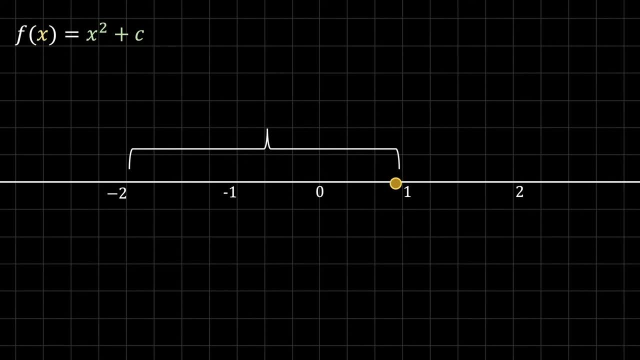 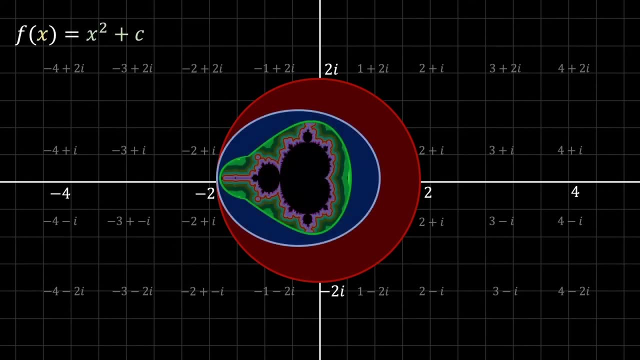 so it is definitely not a bad thing for this function to not grow exponentially here. So we need to learn a couple of more things to understand what just happened. Trust me, learning these things will indeed make it easier for us to understand the subject well. 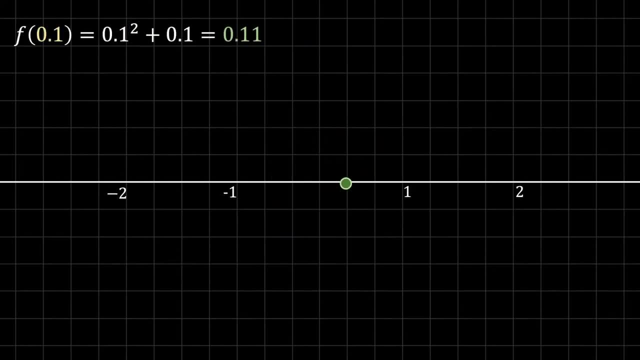 So I want you to focus on an input value which is 0.1, and our output is 0.11.. When we make our input more defined by adding more decimals, we get another output. In this case, it is 0.1596.. 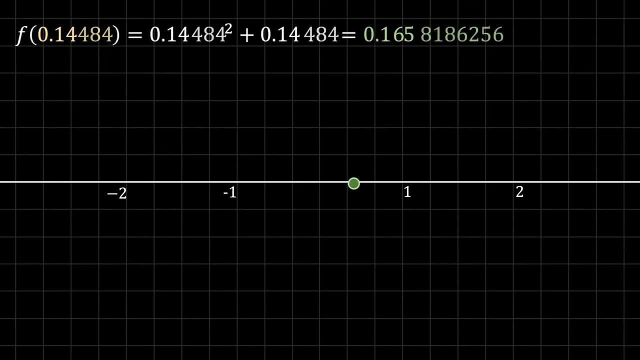 Now let's define our input a lot more by defining more decimals. What we get is an answer which was closer to 0.1.. So let's define our input a lot more by defining more decimals. What we get is an answer which was closer to 0.1. 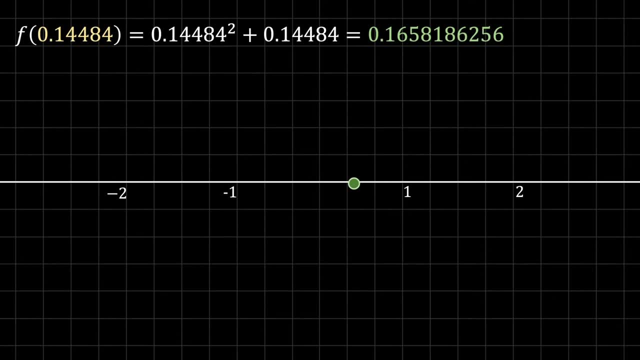 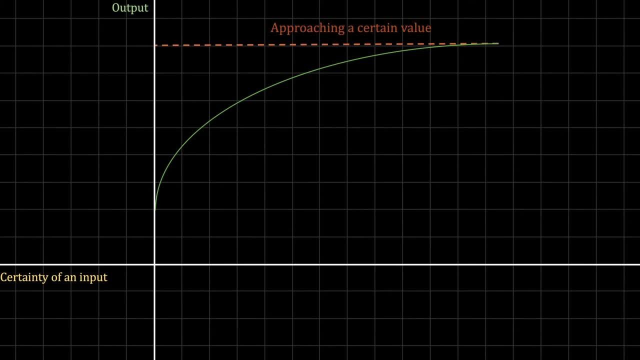 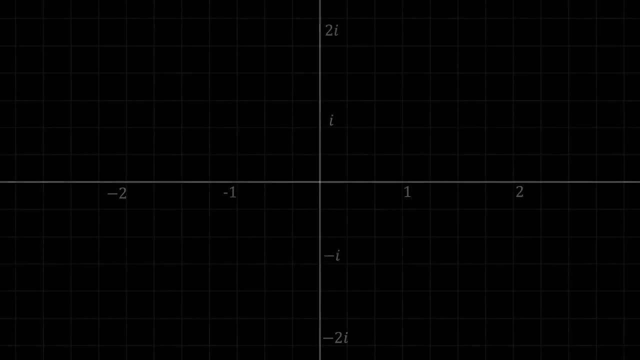 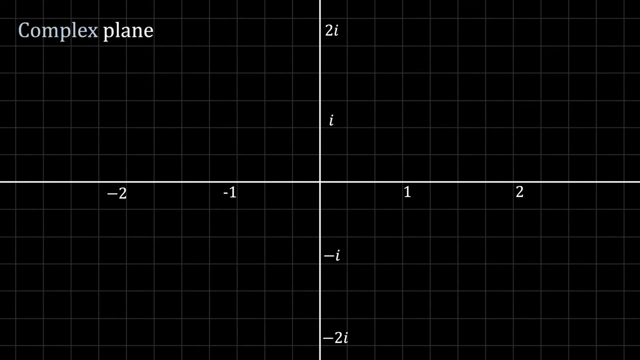 define our input a lot more by defining more decimals. What we get is an answer which was closer to 0.1.. So let's define our input a lot more by defining more decimals. What we get is an answer which was closer to 0.1.. So let's. 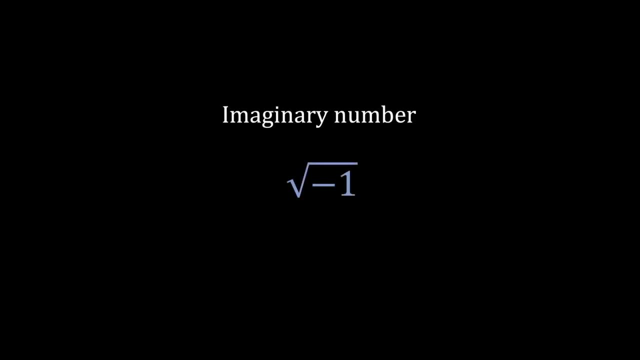 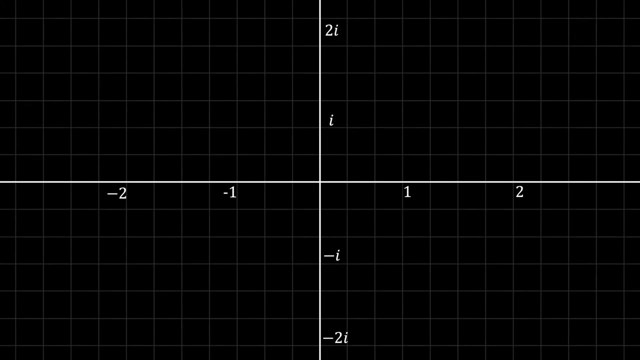 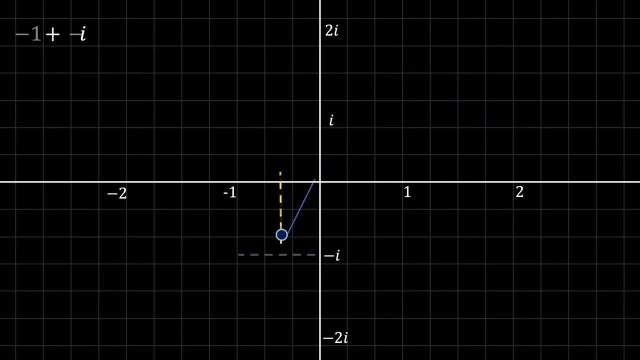 Now let's do something different. We learned how to show these numbers on this plane. Let's do them simultaneously, So let's show a couple of more numbers at the same time as you can see here. For understanding the subject better, I will be showing you another number on this. 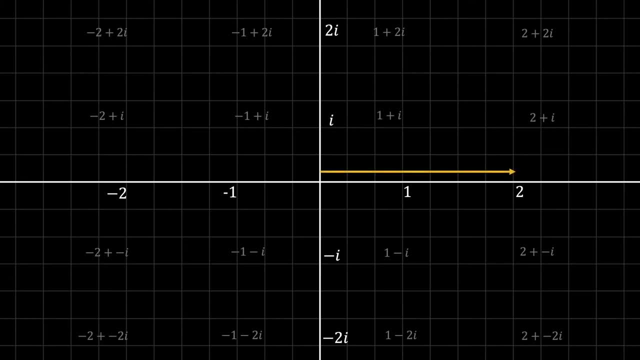 plane. When we go to the number 2 and go 2i above, we end up with, as you can see here, 2 plus 2i. Now, if you remember, the values between these numbers would not exponentially grow. So now let's show these values that would not exponentially grow in the complex plane. 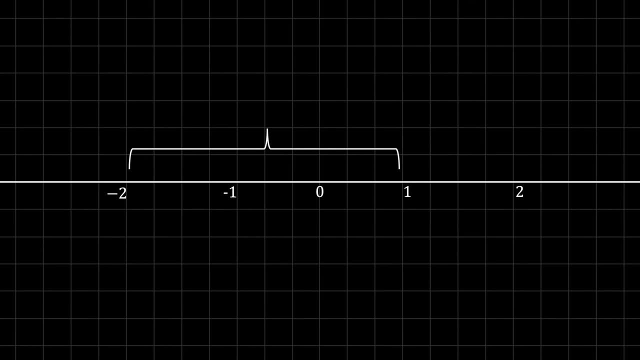 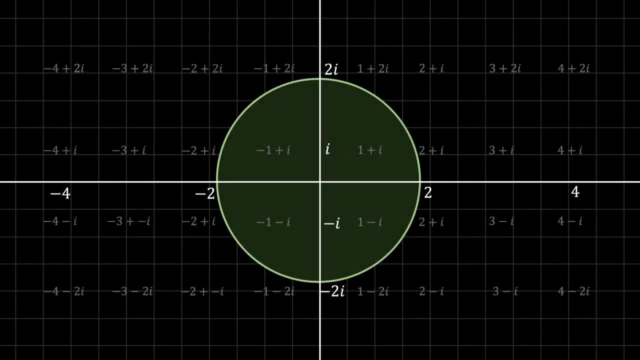 since the normal plane was a one-dimensional, while the complex plane is two, We're going to have something like this: a circle. Values in this area are not growing exponentially, Okay, so now we are going to do something different and interesting. Remember the function that led to this moment: fx equals x squared plus c. 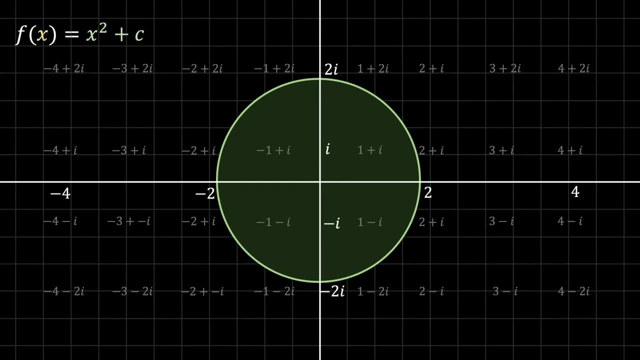 Now let's apply that function to the numbers that are inside of the circle. There is an infinite amount of numbers inside of that circle, but in this graph we can only see 1 plus i. But we know there is more numbers, for example 0.5 plus i and so on, But in this case let's use 1 plus i. 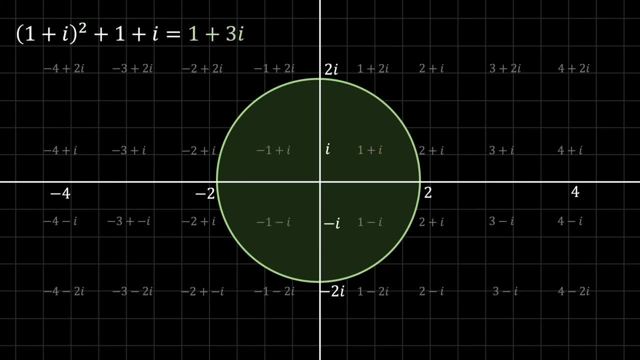 The result is 1 plus 3i. If you check this value, you can see that it's not in the circle. So let's make the numbers that will go outside of the circle red. So if we apply the same rule for all the numbers that are inside of the circle, 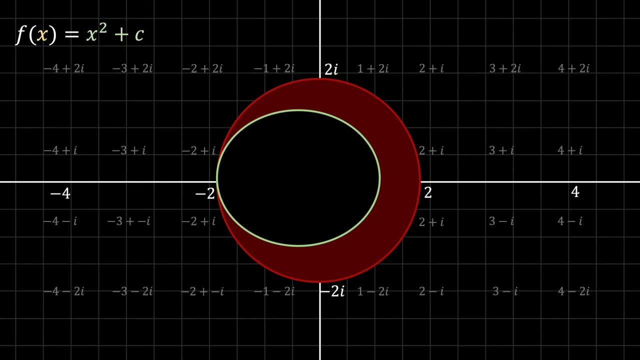 we'll get something like this: Let's apply that same thing to the numbers that are inside of the black zone and colour the numbers that escape from there blue. We will get something like this: Now let's do the same thing again, but now colour it green. We will have something like this: And: 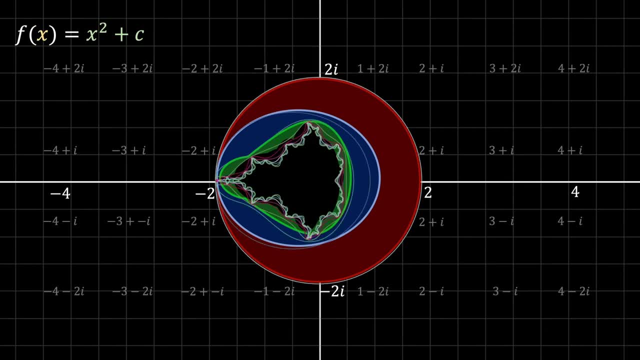 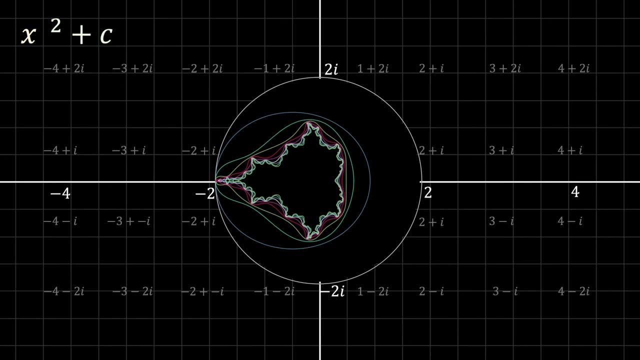 now, if you continue doing this and colour differently, we will end up with this: The Mandelbrot set In literature. this function could be written as not x squared plus c, but z squared plus c, But it makes no difference to the output, so we can continue using our. 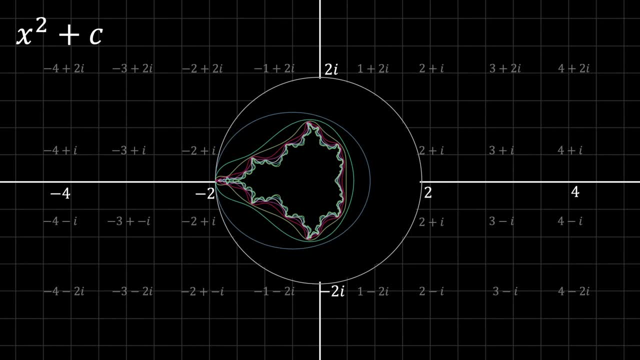 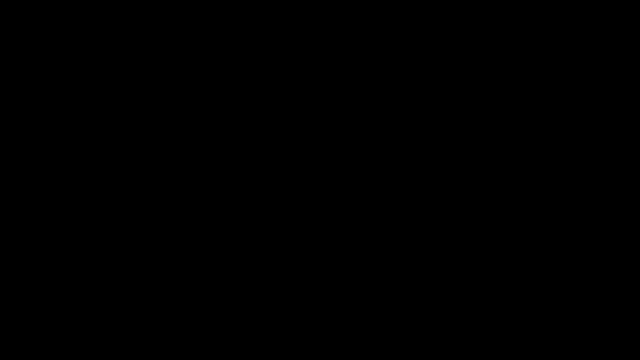 function. This was how to visualise a Mandelbrot set In the next PGA. we shall be talking about its properties and how you can see a part of Mandelbrot set in real life using everyday items. One can see how the lollipop keeps itself clean and held in its shape by hand.